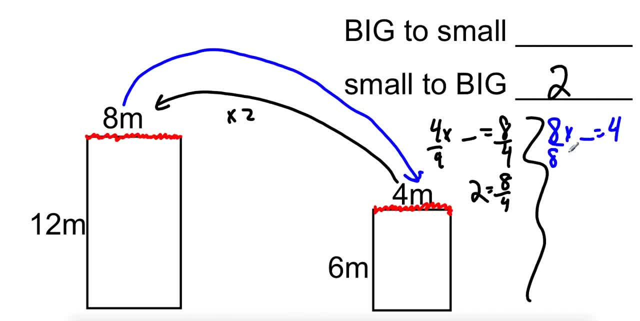 8 times something gives us 4.. We divide both sides by 8, and when we reduce 4 eighths, we get 1 half. Now some of you might be able to identify between these two figures, that these are actually. 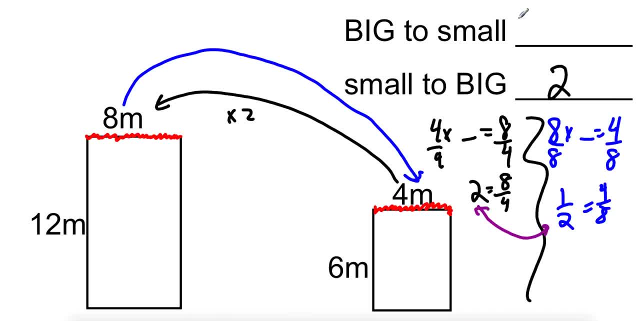 reciprocals of one another. So when finding scales, we're going to be able to identify between these two figures that these are actually. If you know the scale factor going up, you can easily identify the scale factor going down because it's just going to be the reciprocal. So my scale factor from big to small is 1: half and my scale 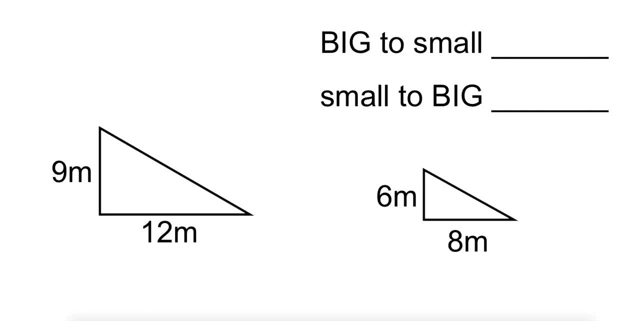 factor from small to big is 2.. In this next example we're going to find the scale factor from big to small and small to big, So we can go from: well, first, before we do that, let's identify corresponding sides. So I can see that 6 corresponds with 9,. 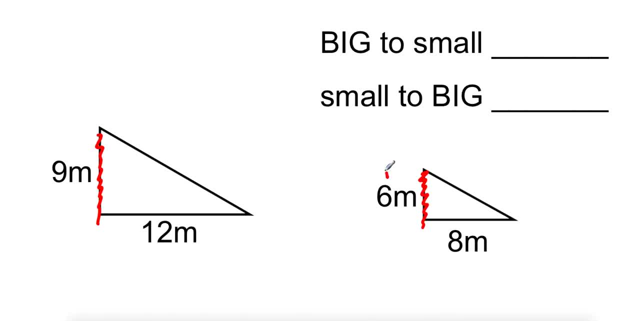 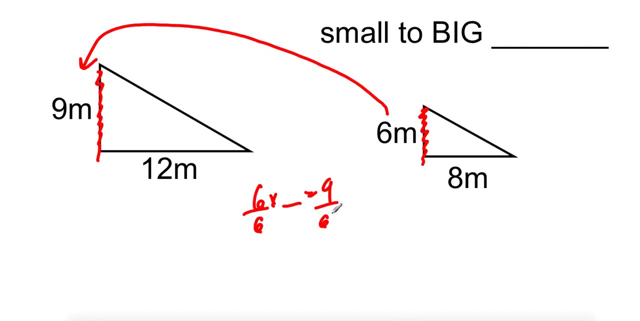 so I'm going to find my scale factor going from small to big. So I know that 6 times something is going to give me 9.. I divide both sides by 6.. 9 over 6 is going to be my scale factor. 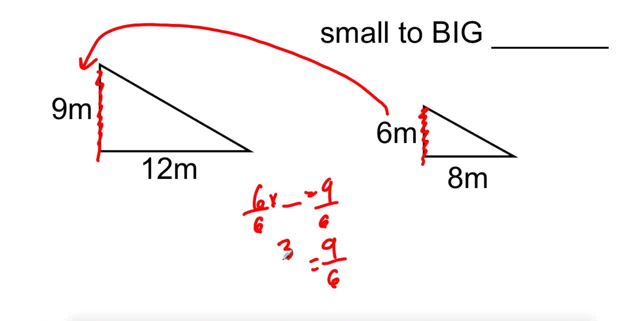 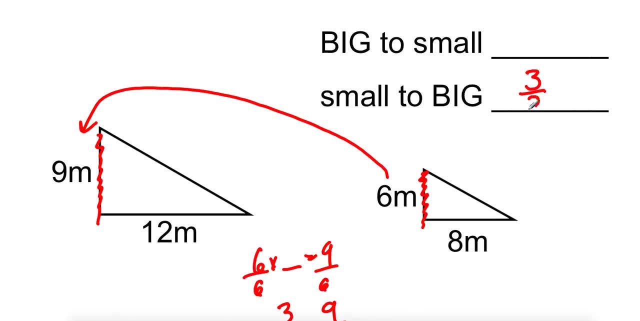 but I can also reduce 9 over 6 by 3 to give me 3 halves. Now that I know my scale factor going from my small figure to my big figure, which is 3 halves, I know that my scale factor going from big to small, this direction is just going to be the reciprocal. 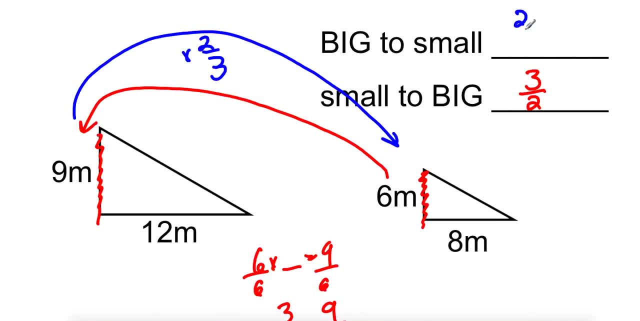 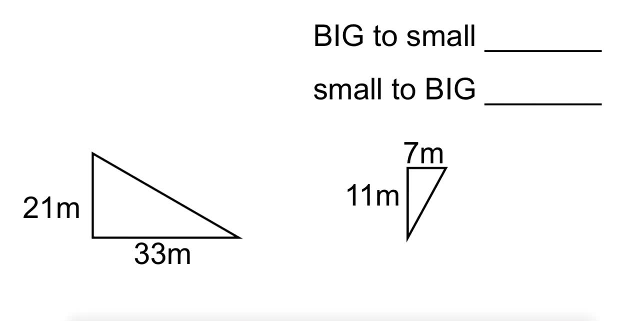 of 2 thirds. Now, in this last example, it's very, again, very important to identify similar figures and corresponding sides. Now I know both of these are similar, so I'm going to find my corresponding side to 11.. Now, 11 is my longer side. This time I'm going to go for my longer side. 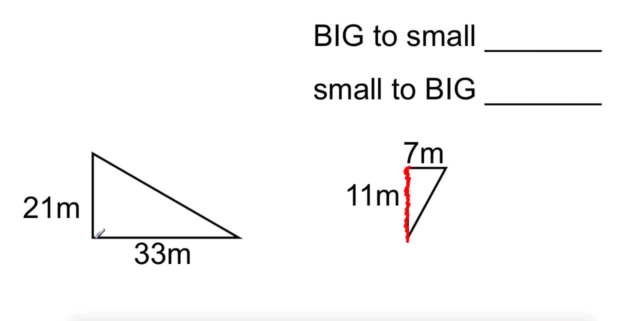 And I can see that 33 is my longer side over here, So I'm going to compare. this time I'm going to go from small to big. I'm going to go this direction. I'm sorry, big to small. Let's go this direction this time.